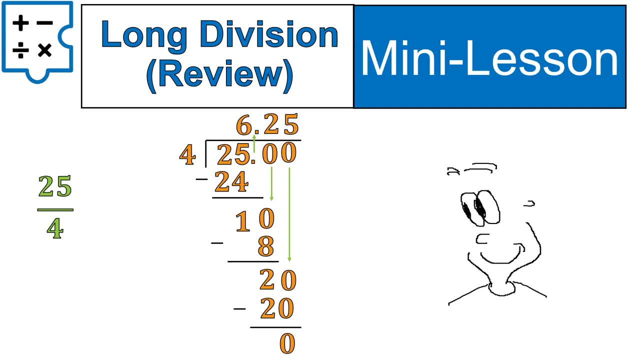 The decimal goes right there and that's our final answer. So this is long division with finding decimals. It's basically the next step after finding remainders, And everything that we're going to do today has to do with long division and decimals. 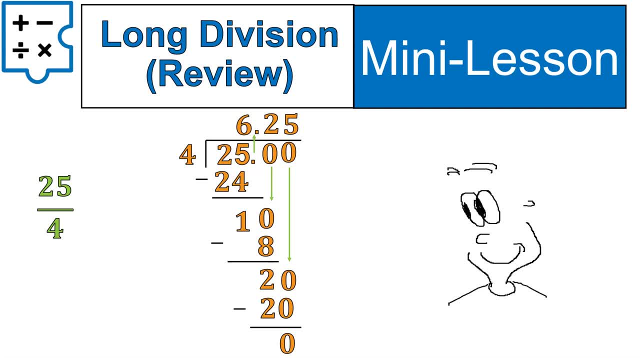 So if you've never seen this video, please check it out. If you've never seen this before, I would check out a video on that first, But if you have seen this before, I apologize for this 2 minute long review. you did not need. 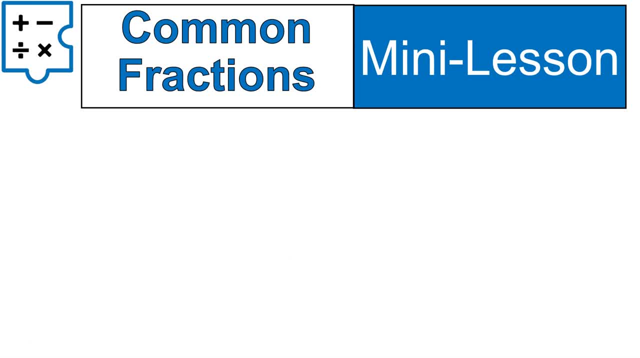 Let's go ahead and get looking at a couple of common fractions and then we'll get into repeating and terminating. First off, this is a common fraction: 1 half. Inside your head, you might already know what this is as a decimal, but I'm going to show you real quick how you would calculate it. 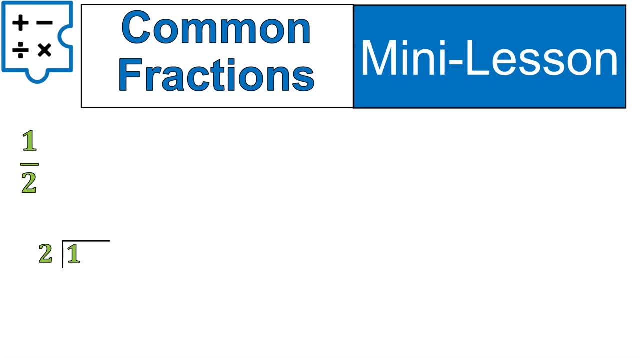 You would write it out like this: How many 2's are there inside of 1? There's none. so now we're going to add that point 0,, like we did in the previous example. That decimal goes there. How many groups of 2 inside of 10? Well, there's 5.. 5 times 2 is 10.. We get a 0, and our answer is 0.5. 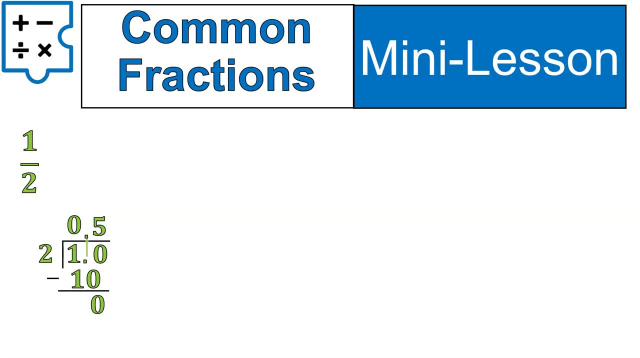 You might have already known that 1 half was 0.5, but that is why and that's how we do the division. to find it, Let's do another couple: 1, fourth, or 1 divided by 4.. We'll put up that 0.. 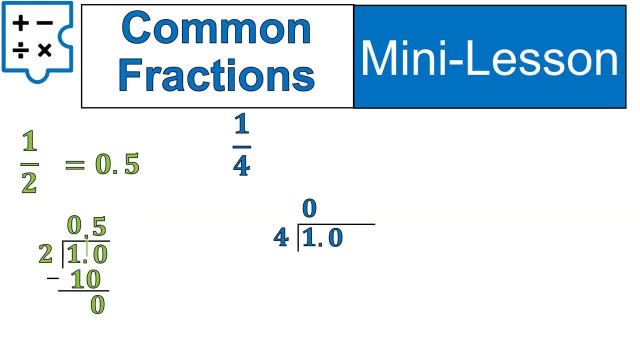 We'll throw up there because there's no groups of 4 inside of 1.. We'll add that 0.0 there, knowing that we need that decimal to line up. Now let's pretend the decimals don't exist and say how many groups of 4 inside of 10.. 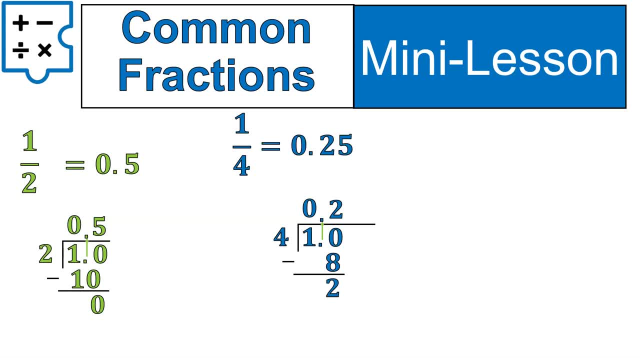 Well, there's 2.. We multiply, subtract and bring down a 0, subtract for our final answer. So that's what you get: 1 fourth is 0.25.. Again, A common fraction that you've probably seen before. 1 quarter is 0.25.. 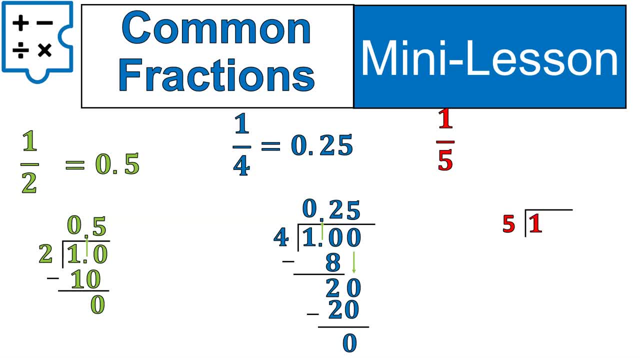 Let's do one more. that's maybe not quite as common as the first two, but we'll solve it the same way. We ask how many groups of 5 inside of 10.. Well, there's 2.. 2 times 5 is 10.. 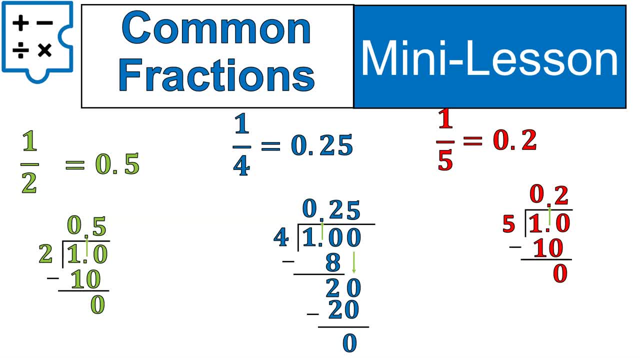 And so we get a nice even 0.2.. So here's what we have: 1 half 0.5, 1 quarter 0.25, and 1 fifth 0.2.. All of these are examples of terminating decimals. 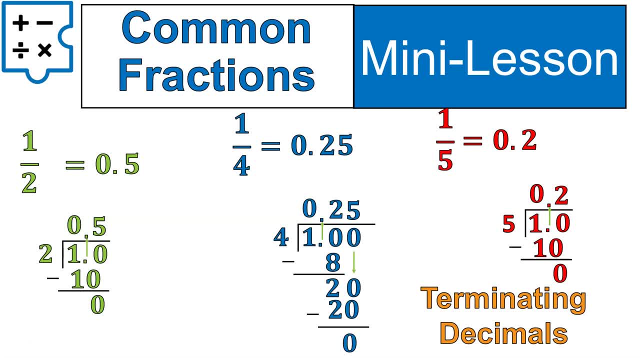 They're also very common fraction-to-decimal conversions, So those are ones that you want to keep track of. We call them terminating decimals because they stop Right, They end, They eventually get a 0 remainder. That's what a terminating decimal is. 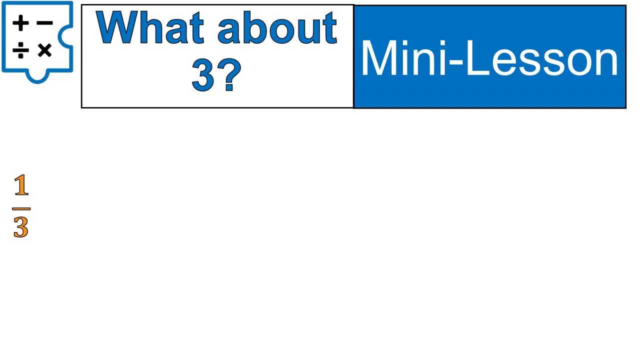 What about when we get the number 3, like 1 third? This is also a common fraction, but it's a little bit different. Let me show you. Let me show you what happens when we divide this Again. we can't fit. There's no groups of 3 inside of 1.. 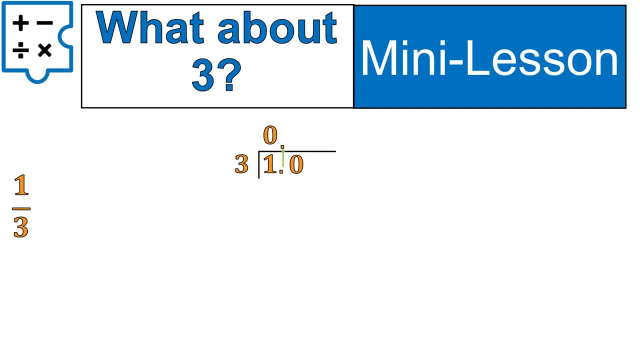 1 is smaller than 3.. So we're going to move along. How many groups of 3 inside of 10?? Well, there's 3 of them. 3 times 3 is 9.. And when we subtract we get a 1.. 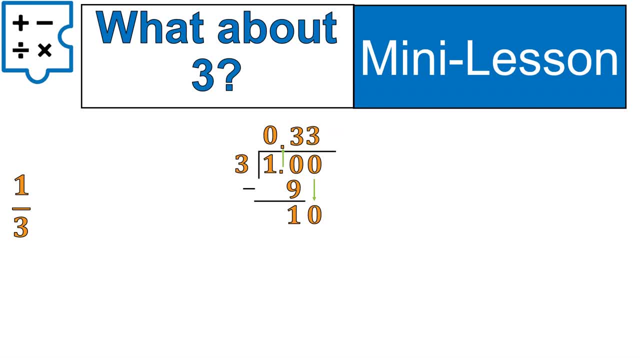 Now you may notice a pattern here. Now, how many 3s inside of 10?? Well, there's 3.. 3 times 3 is 9. And that leaves us with 10.. You notice that this is a pattern that will continue forever. 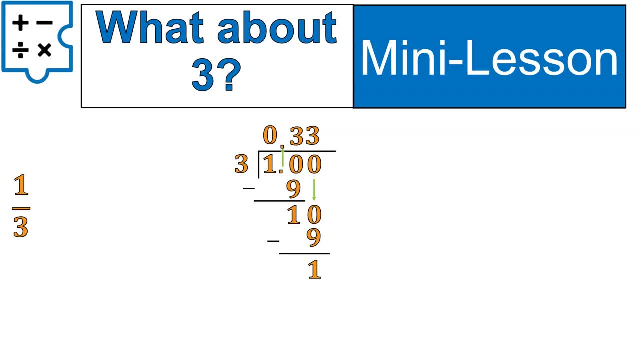 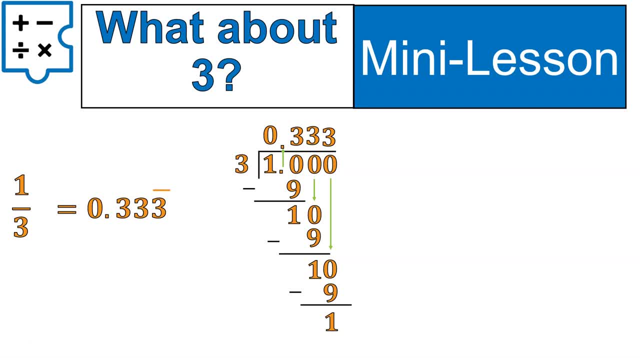 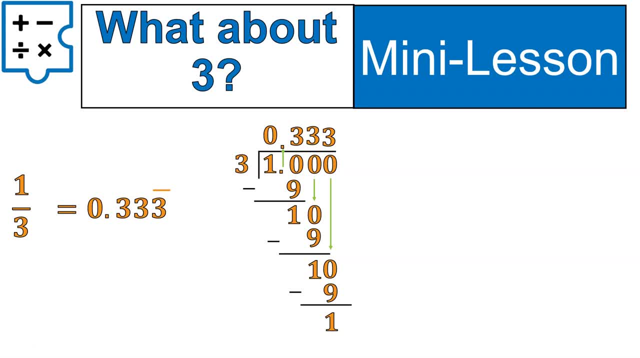 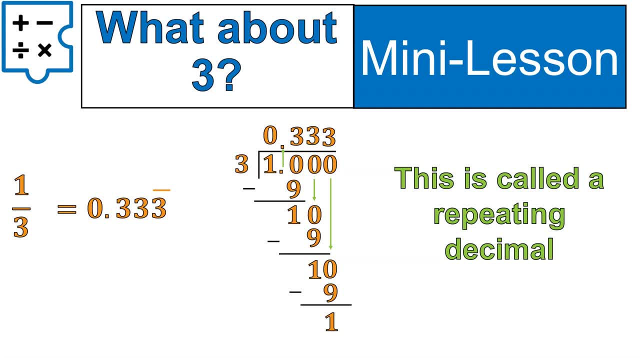 Notice that this is a pattern that will continue forever. So there are two types of decimals we're talking about today: repeating decimals and terminating decimals. Okay, terminating decimals. stop repeating decimals continue to repeat over and over and over. They may repeat one number like this, or they might have a repeating pattern, but either way, they repeat infinitely. 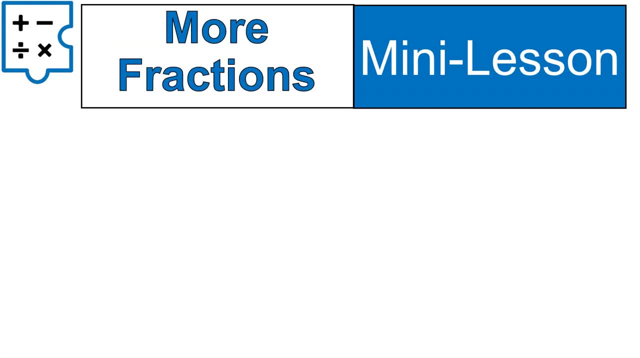 So we use that line to kind of indicate that: Alright, here are a couple more fractions. We've got two-fifths, which is two divided by five, and we would solve it in this way and get 0.4.. That's another example of a terminating decimal. 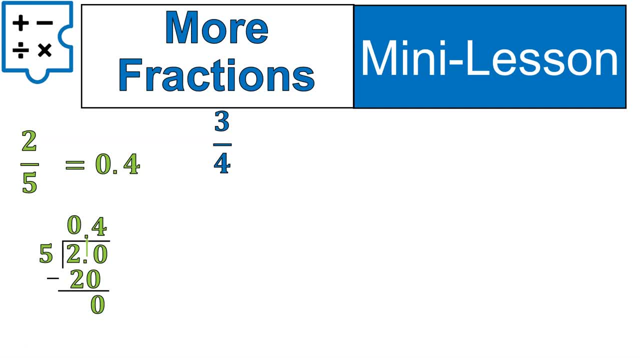 I want you to try this one out three-quarters, Set it up and solve that one as a division. question Three: two, one go. Hey, welcome back. This might also be one that you're familiar with, Because three-fourths or three-quarters is equal to 0.75, so you might have already solved this type before. 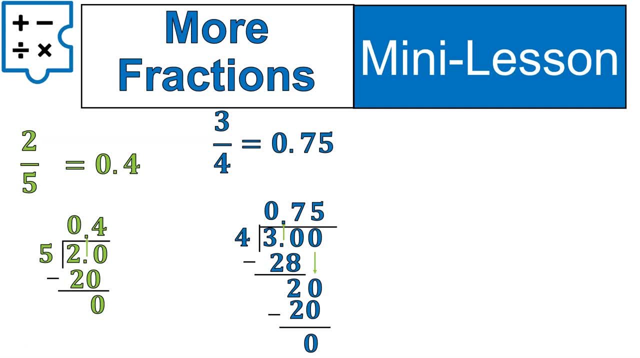 If not, there are the steps of how to solve it using long division. Here's another one, two-thirds. I want you to try that one out and see what happens. Go for it, Alright. that one was a little bit more tricky because this one is a repeating decimal. 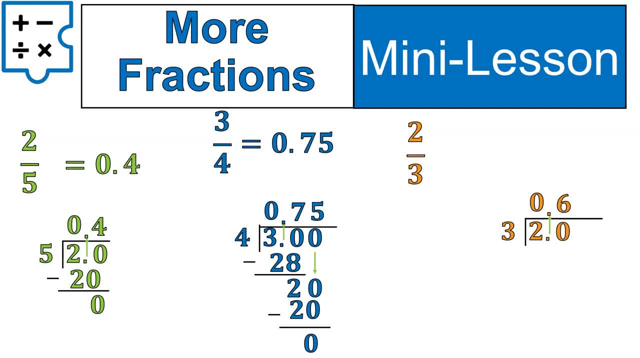 There's no groups. We've got groups of 3 inside of 2.. But there's 6 groups of 3 inside of 20.. It's 18, so we'll subtract, Add another 0, and we get 18.. 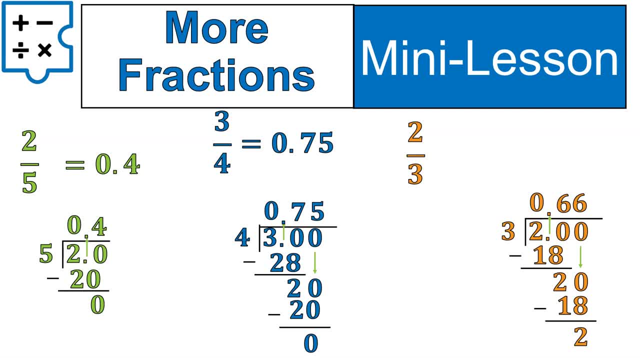 We repeat that process over and over. There's always going to be 6 groups of 3 inside of 20.. When you subtract, you always get a 2. When we bring it down, that'll become 20.. The process will repeat. 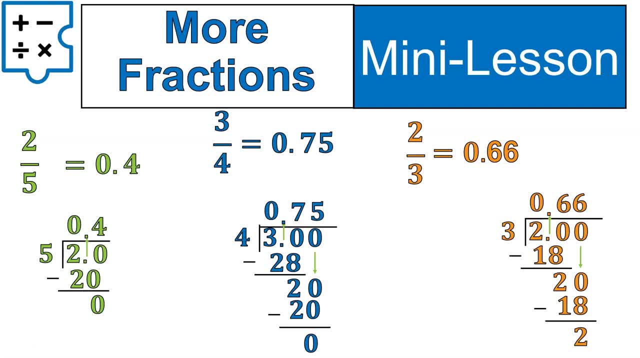 If you solve that one using long division, you know what you're going to do. Yes, sure You know that. Sorry, Let's go right to it. know that 2 thirds is 0.66 and we say that 6, 6, repeating, we can draw that line. 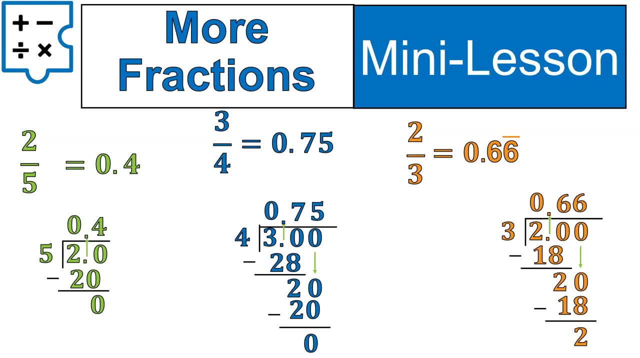 over top of the 6, because that is the part that's repeating, than just a single digit of 6 is repeating over and over and over, forever. all right, so that is repeating and terminating decimals. it's a very common thing. all repeating or terminating decimals can be written as fractions. all right, so we call them. 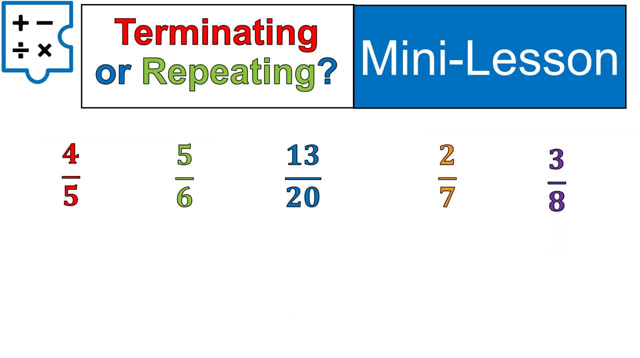 rational numbers, they're repeating or terminating decimals. now there is a quick way that you can tell if they are terminating or repeating, and this is the shortcut that I talked about in the introduction. all right, okay, I'm gonna race and we're going to determine whether these are terminating and 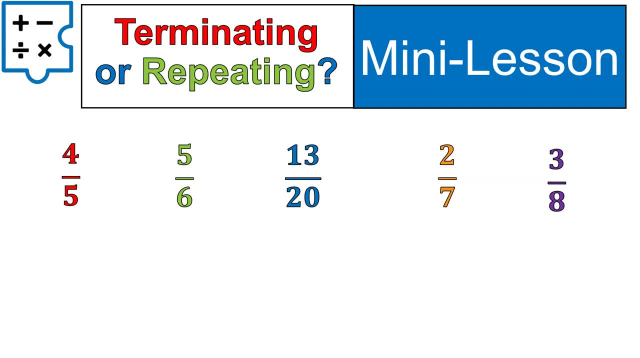 repeating, so I want you to use the old method. that's super slow. you do long division on all of these and I will do my quick, short method and we'll see who can do it faster. three, two, one go. bing, bing, bing, bing, bing, done. well, that's not fair. I had all the answers. 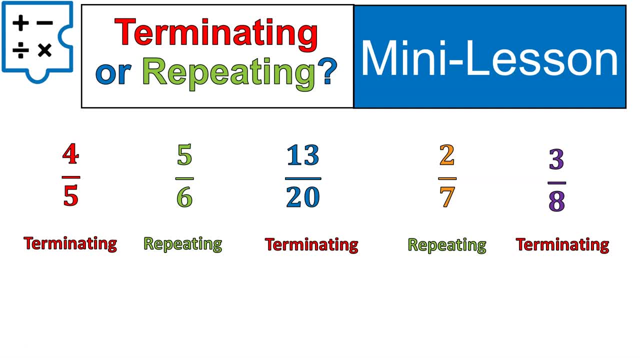 that is very true. I did have the answers, but you can solve it almost this quickly if you know the shortcut. let me tell you the shortcut and then I'll show you how it works. the shortcut is really: there's only two numbers that give you terminating decimals: twos and fives. 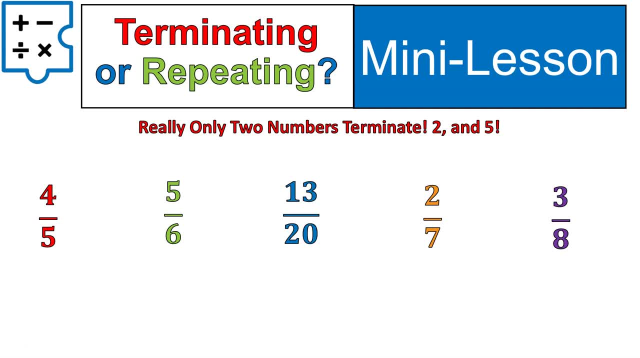 and if you find the prime factorization of any of these numbers, and they're made up of only twos and fives, then you have yourself a terminating decimal. let me show you an example. so if we look at our first fraction, four over five, that one. 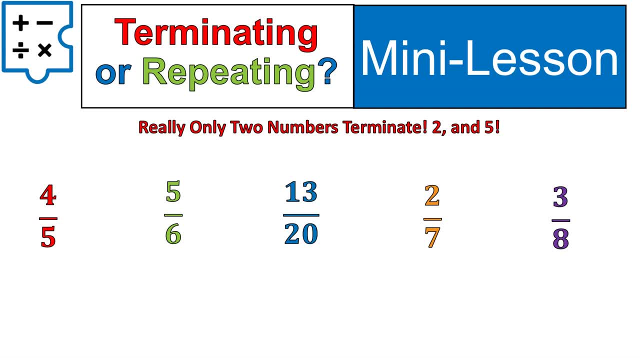 has a five, its prime factor is five. right, the? that's the only prime factor of five is five. therefore, this one is terminating, so you terminating. the prime factorization of six is two times three. so although it does have a two in it, it's. it also has a three, which is a repeating decimal. 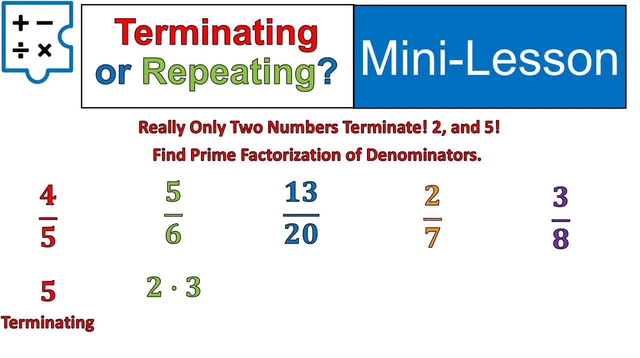 number. it is not made up of only twos and threes, therefore twos and fives. I'm sorry, so therefore it's repeating. let's look at the number twenty. twenty in prime factors is two times two times five. that is made up of only twos and fives. 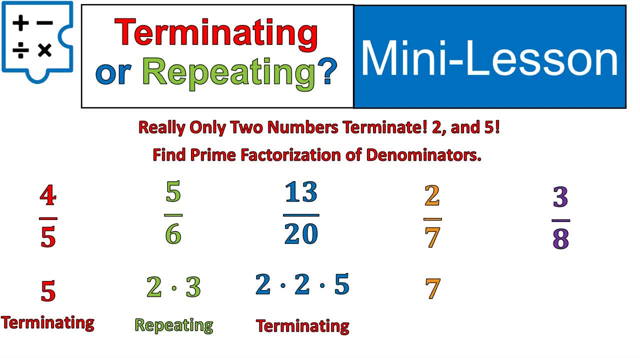 therefore it is a terminating decimal. seven is a prime number, not a two or five, therefore it's a repeating decimal. and three over 8? 8 as a prime factor, is two times two times two. those are all factors of either two or five. therefore it's a terminating decimal. so you can figure this out using just the.